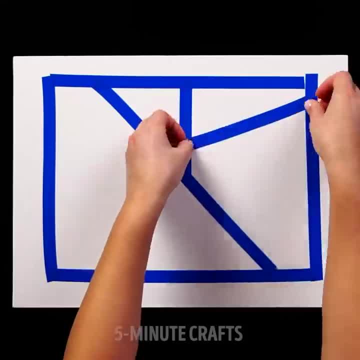 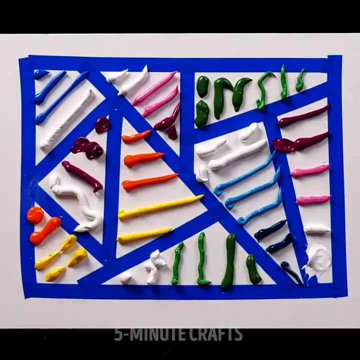 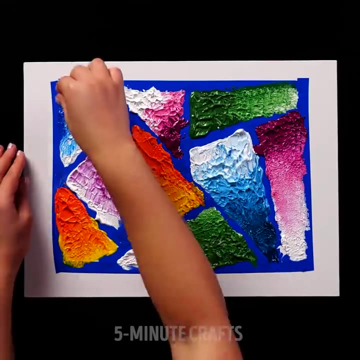 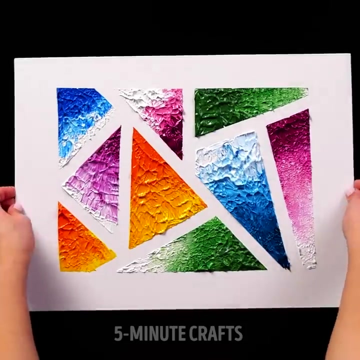 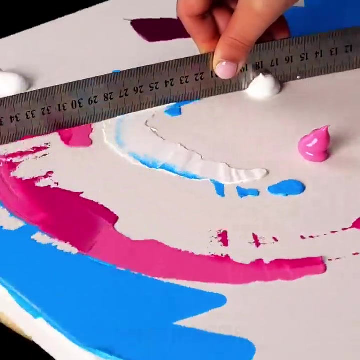 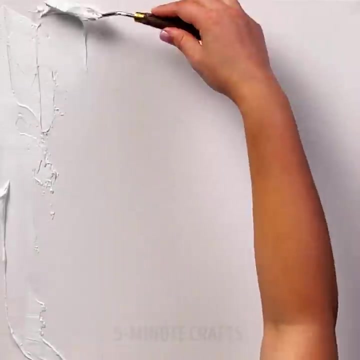 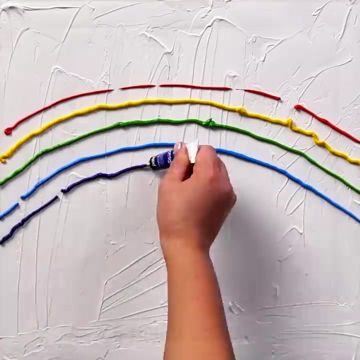 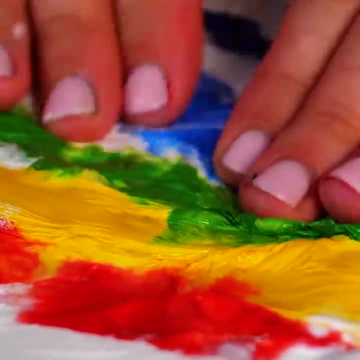 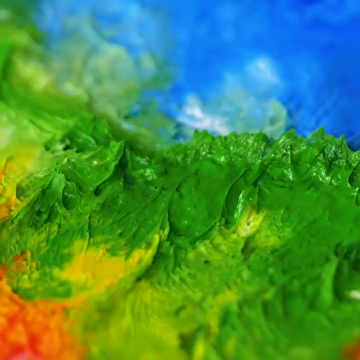 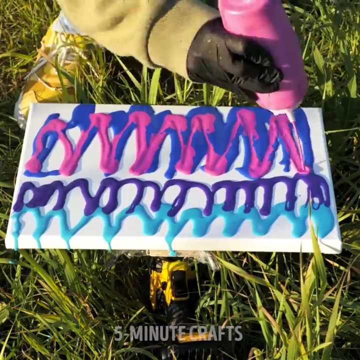 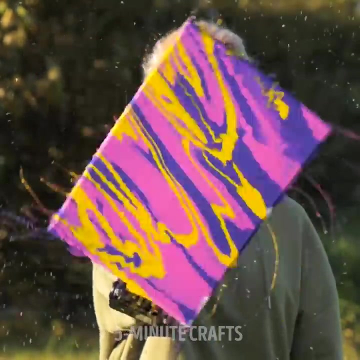 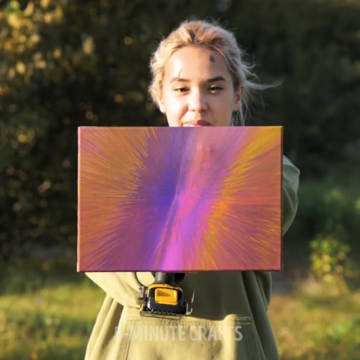 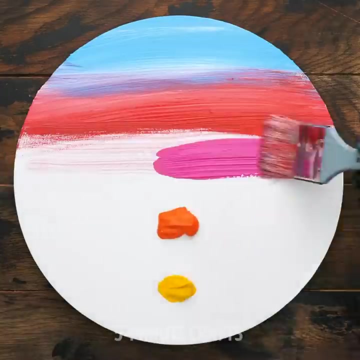 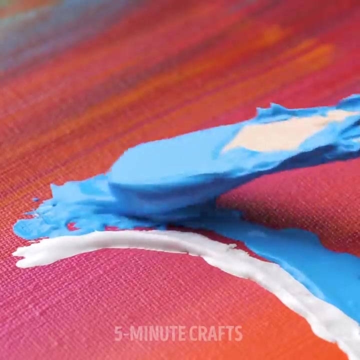 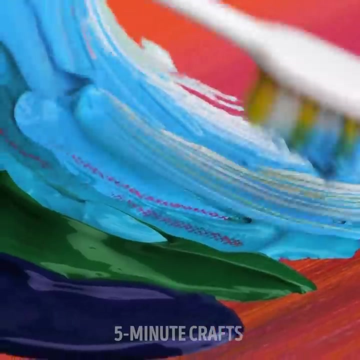 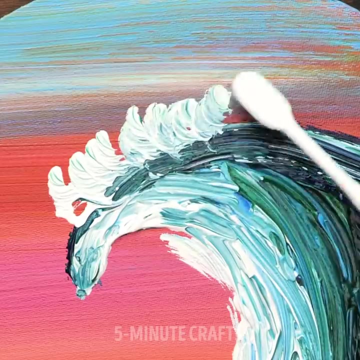 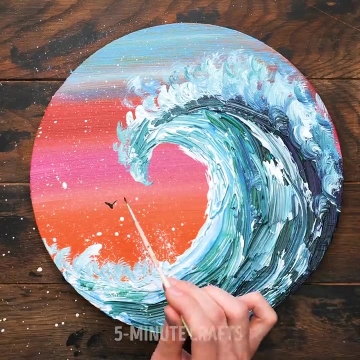 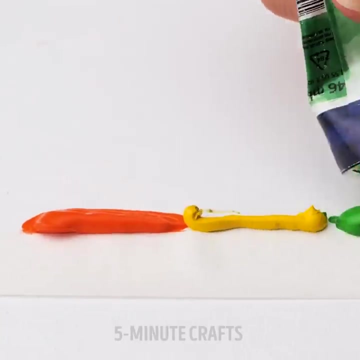 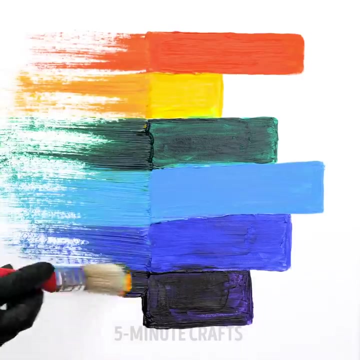 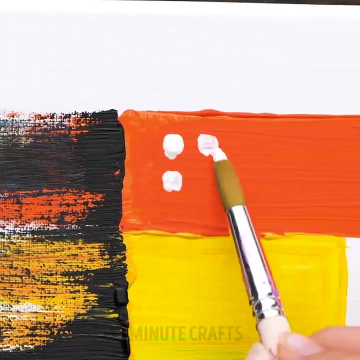 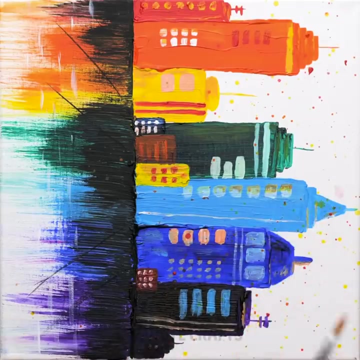 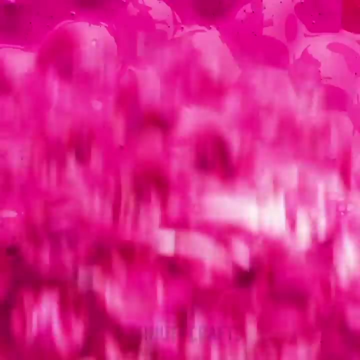 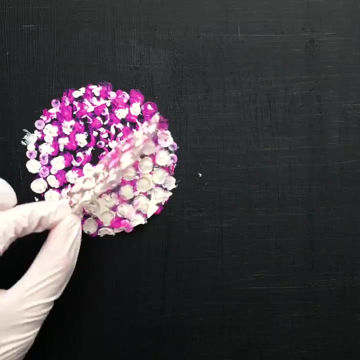 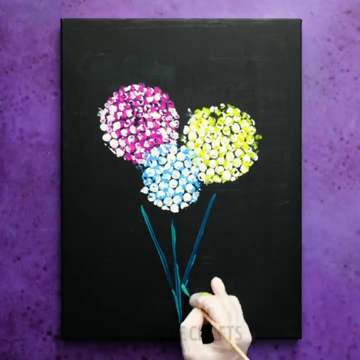 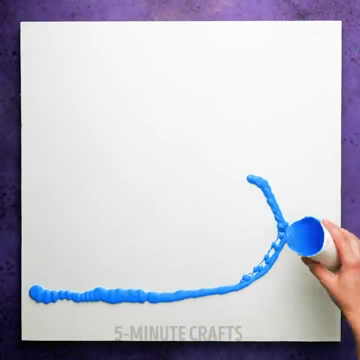 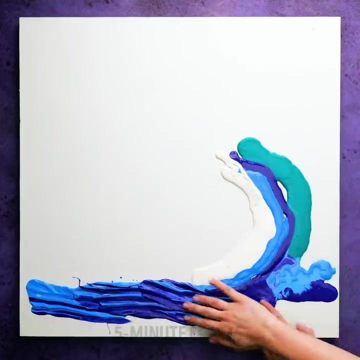 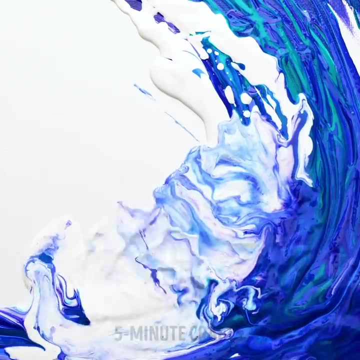 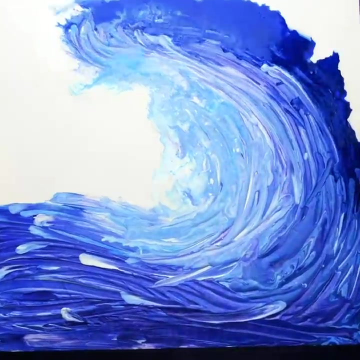 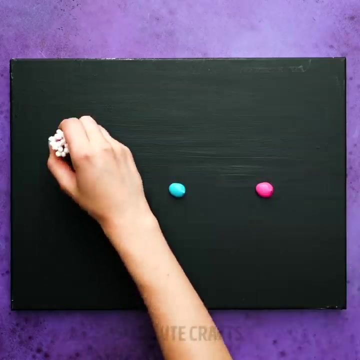 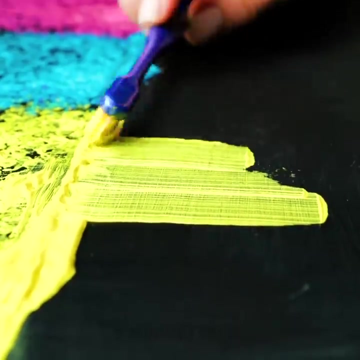 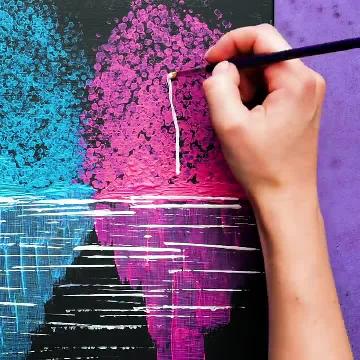 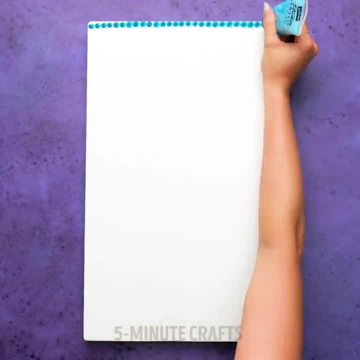 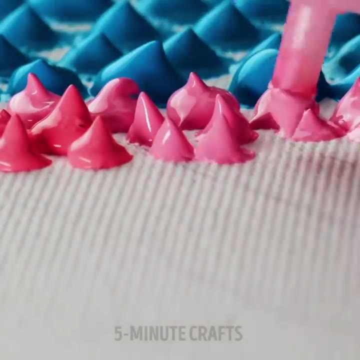 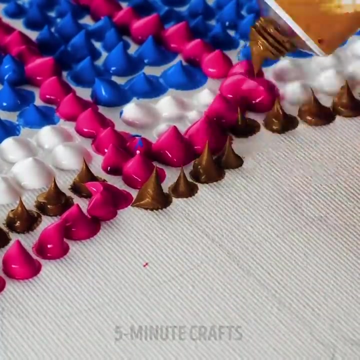 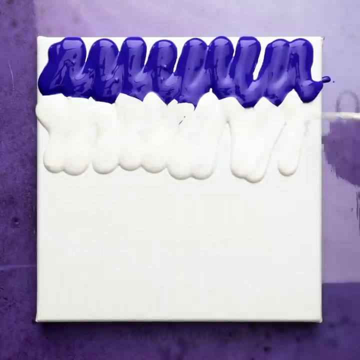 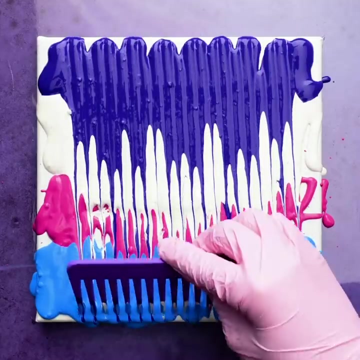 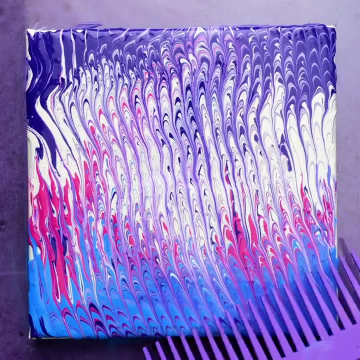 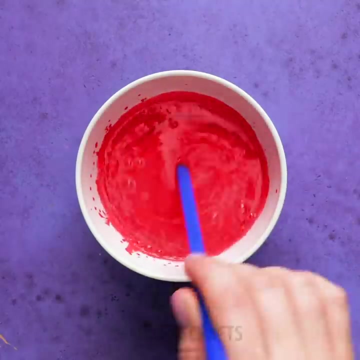 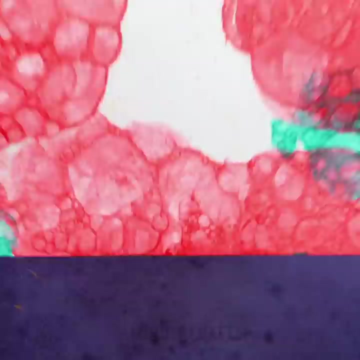 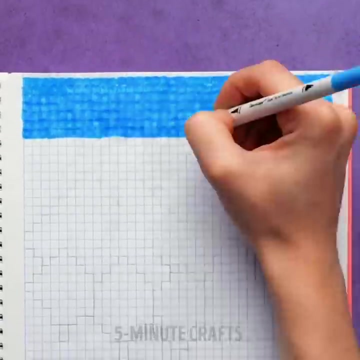 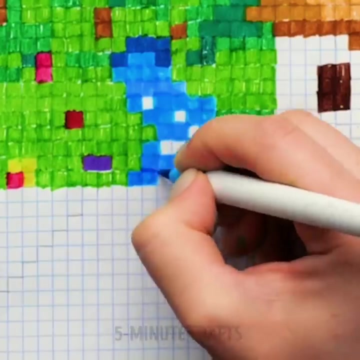 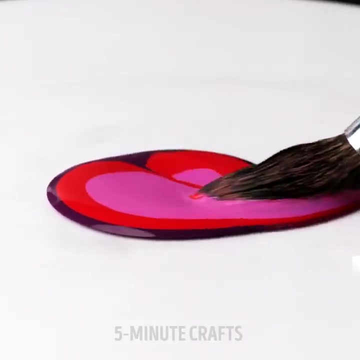 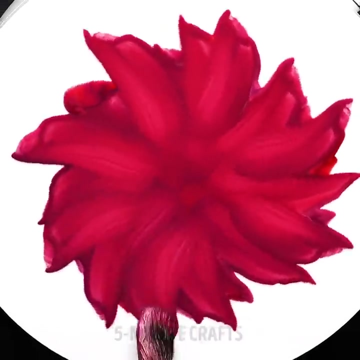 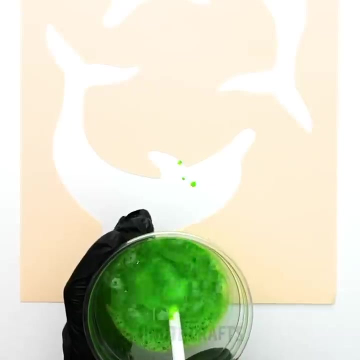 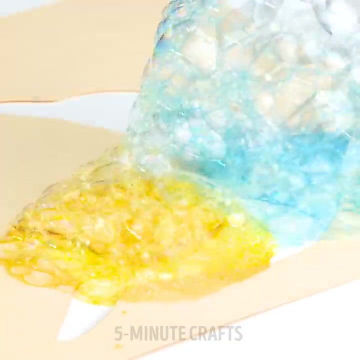 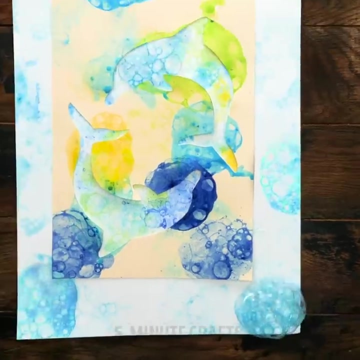 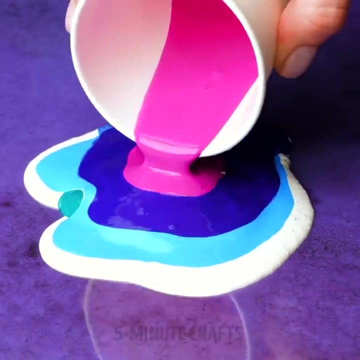 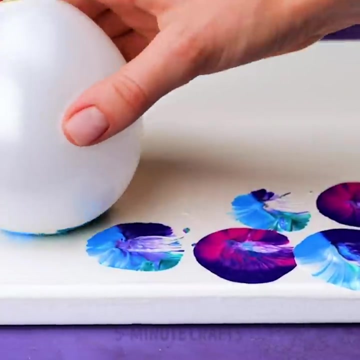 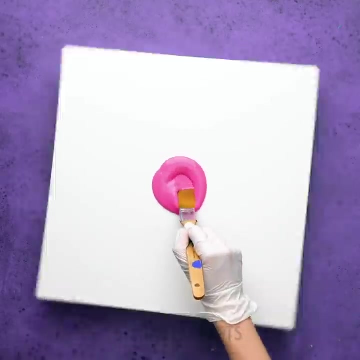 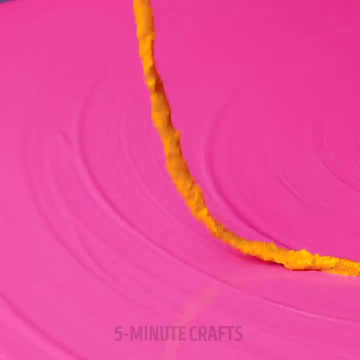 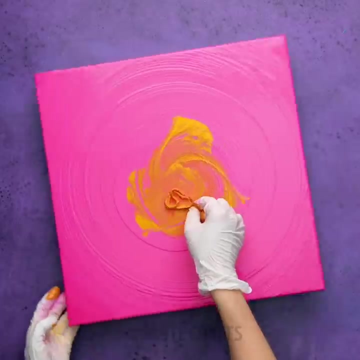 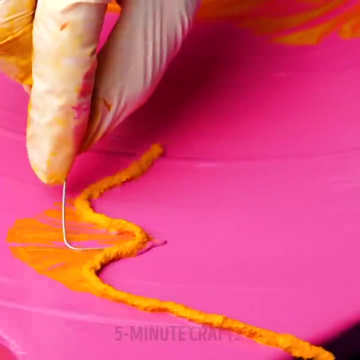 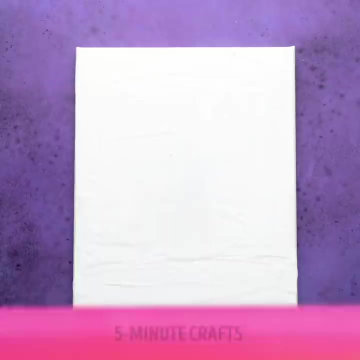 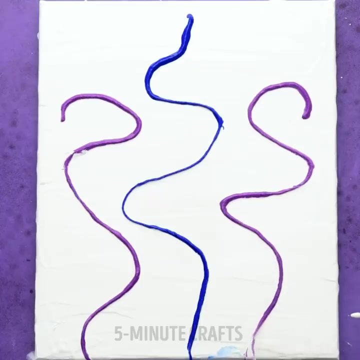 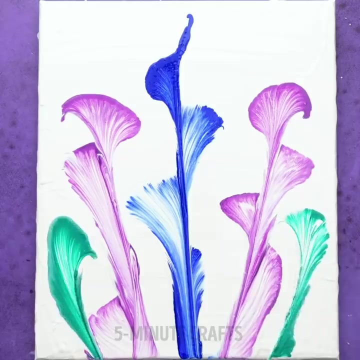 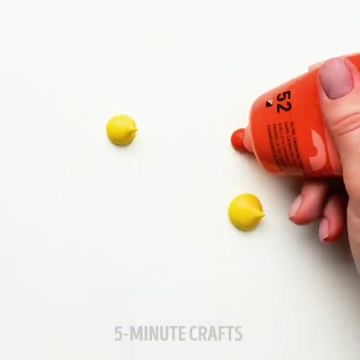 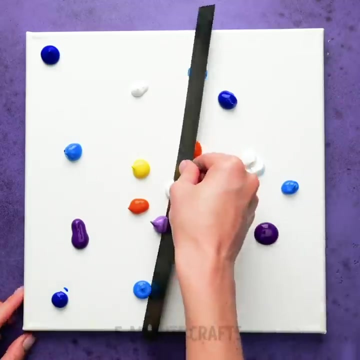 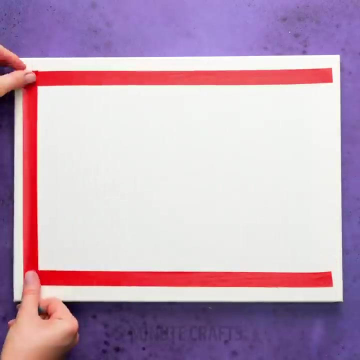 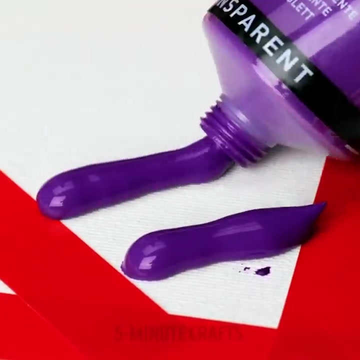 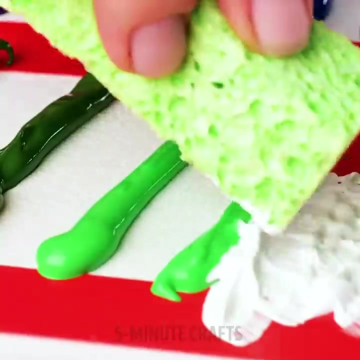 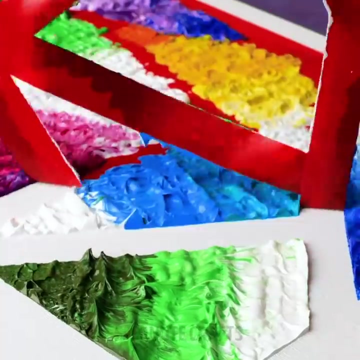 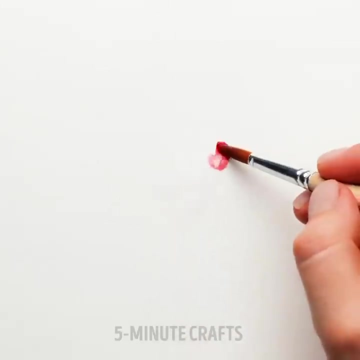 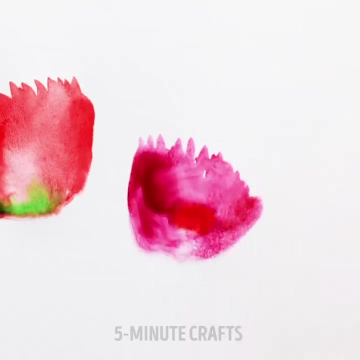 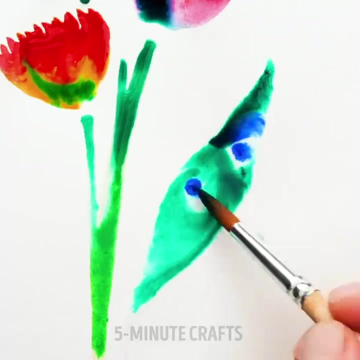 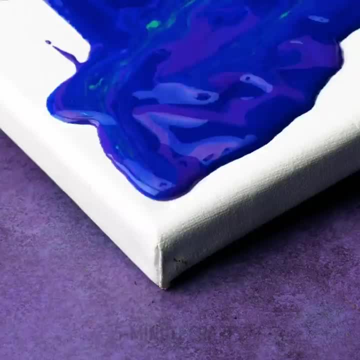 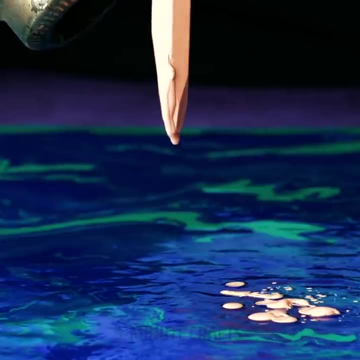 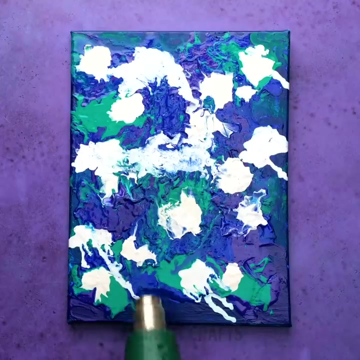 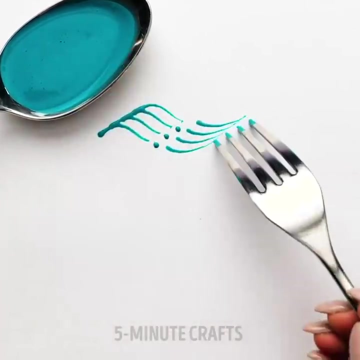 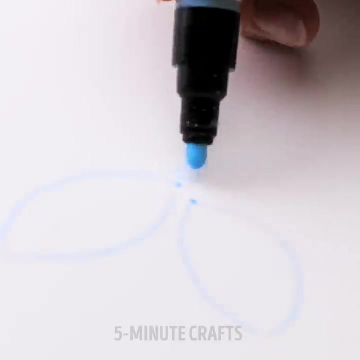 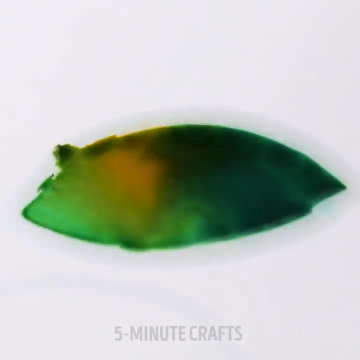 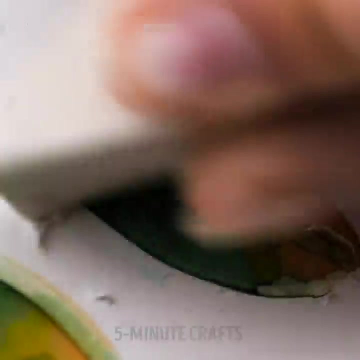 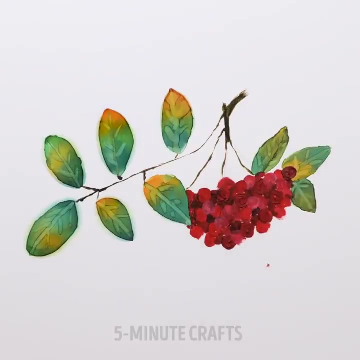 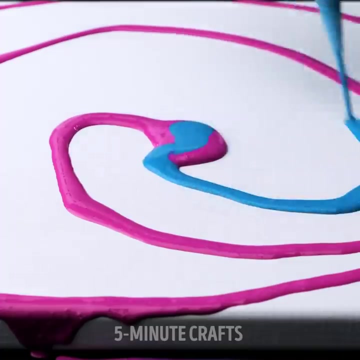 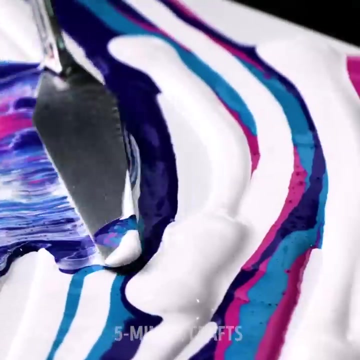 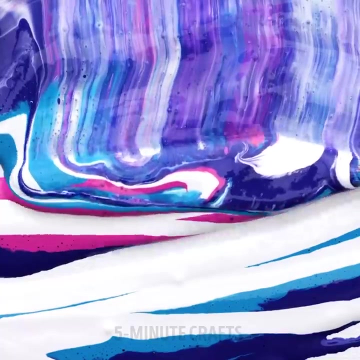 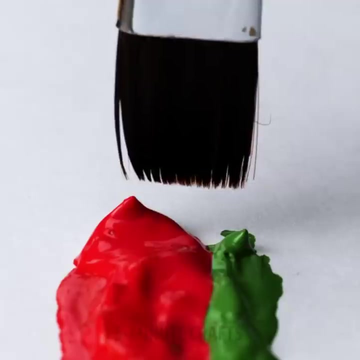 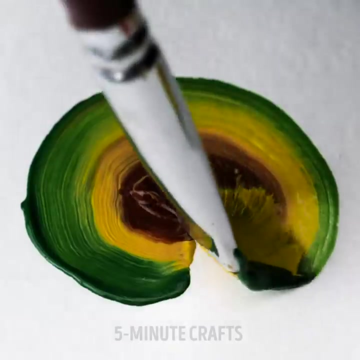 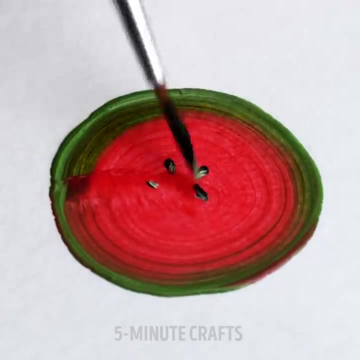 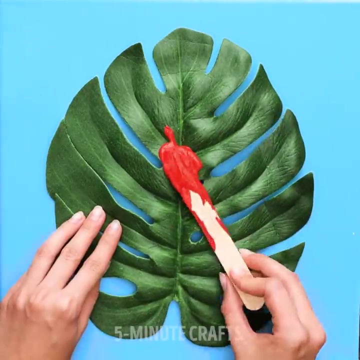 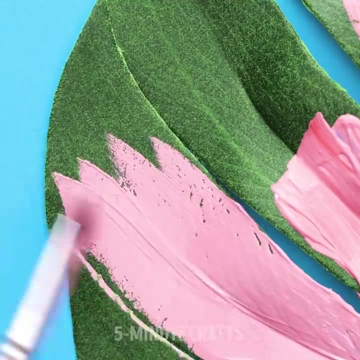 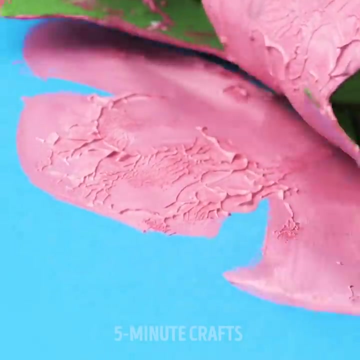 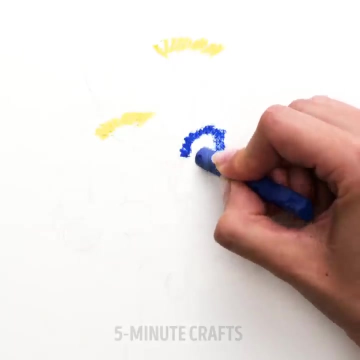 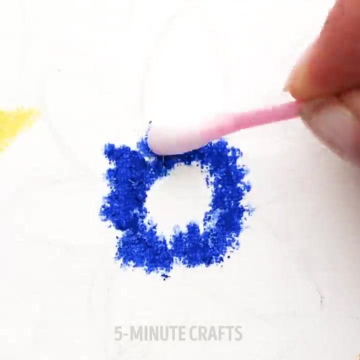 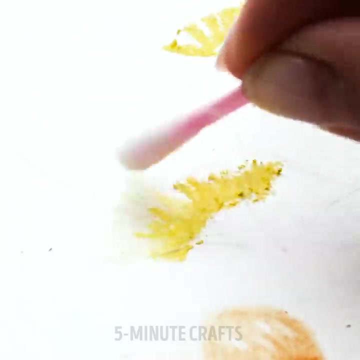 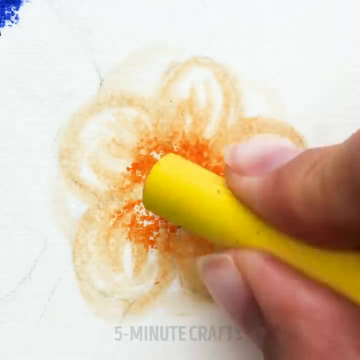 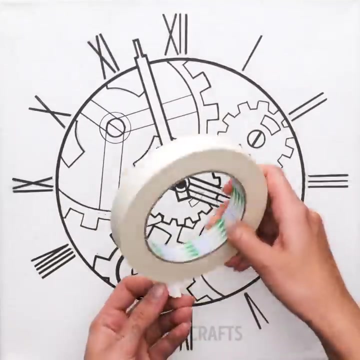 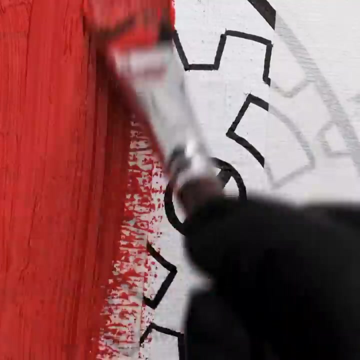 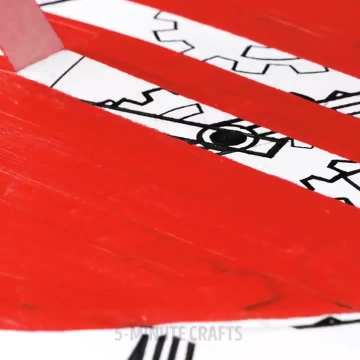 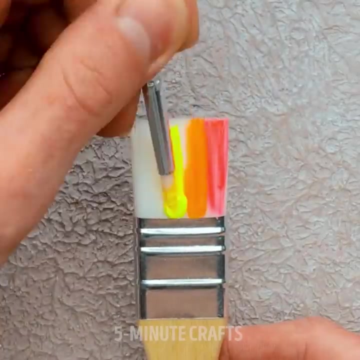 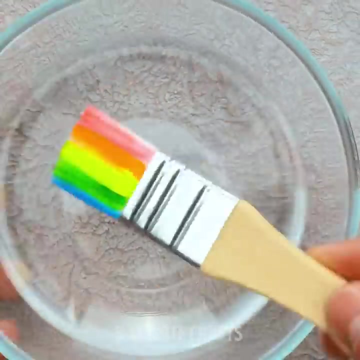 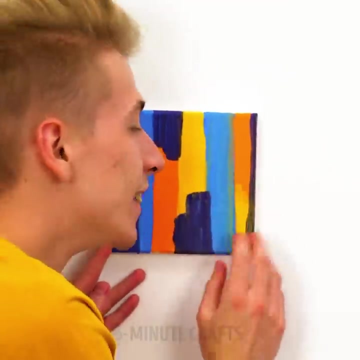 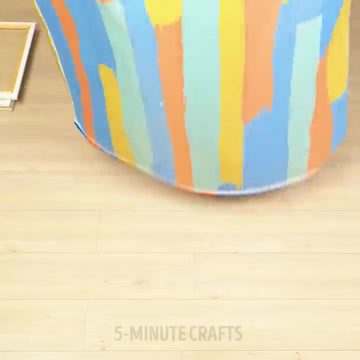 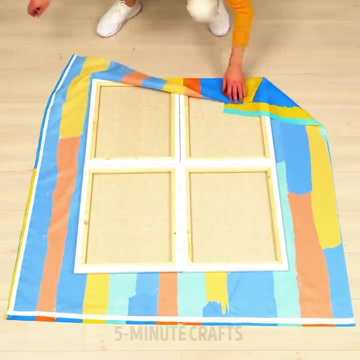 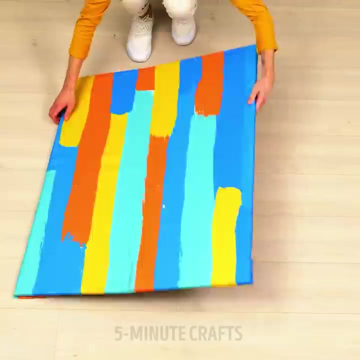 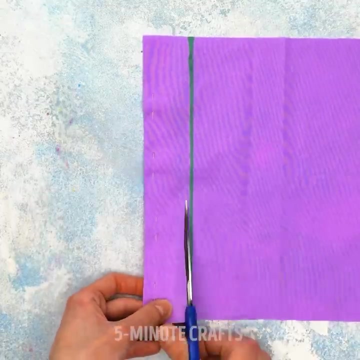 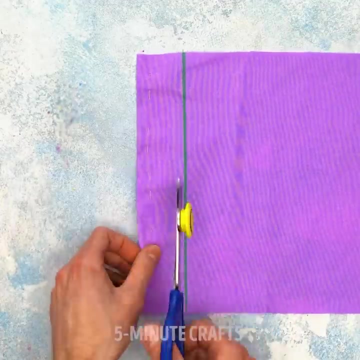 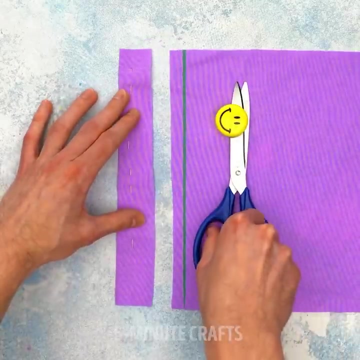 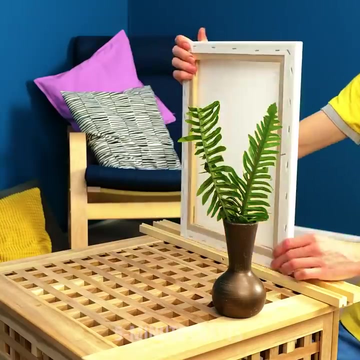 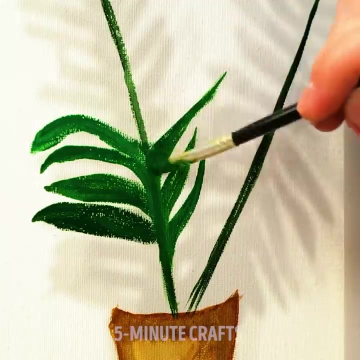 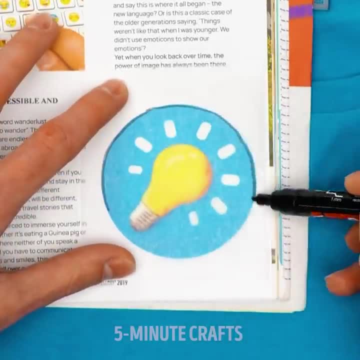 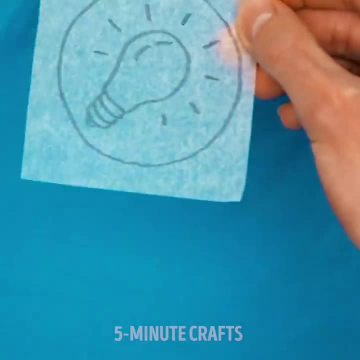 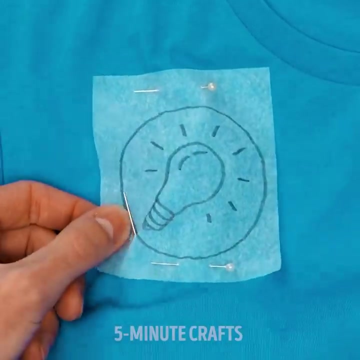 But I don't wanna be the one to say, oh, I told you so. And even if the sky was falling down, You never noticed anyone around. I don't wanna be the one to say, oh, I told you so, But I told you so. 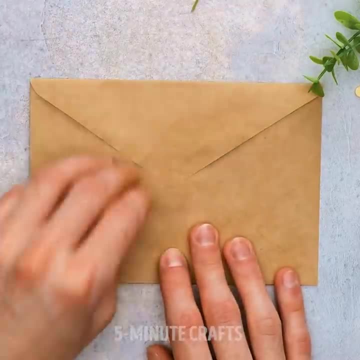 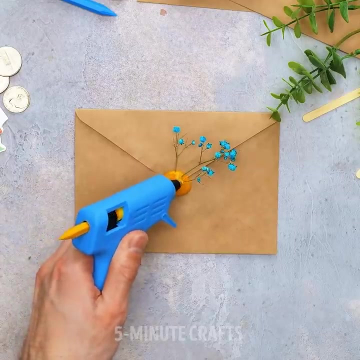 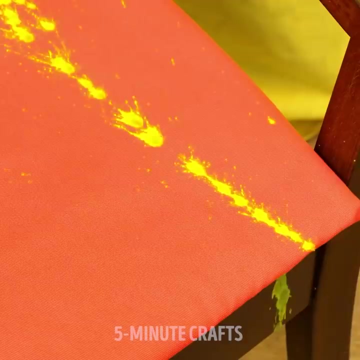 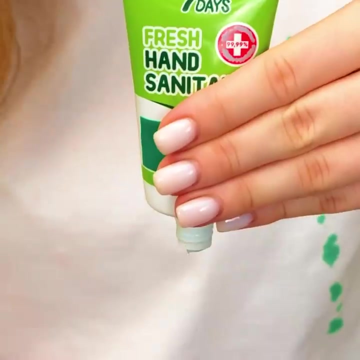 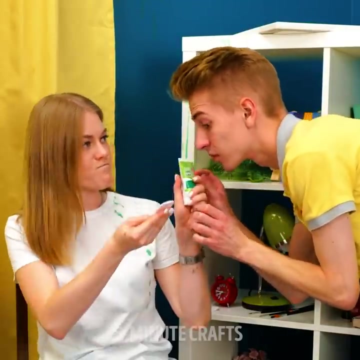 Keep on acting out like strangers. Scream out loud: I will go if nothing changes. So change your heart. Ooh, your mind is a ghost town. Ooh, your mind is a ghost town. Ooh, your mind is a ghost town, Echoing inside your walls. Five feet underground now. Nothing's gonna save us from our doubts, Nothing's gonna make us spell it out. I don't wanna be the one to say, oh, I told you so, But I told you so. I don't wanna be the one to say, oh, I told you so. 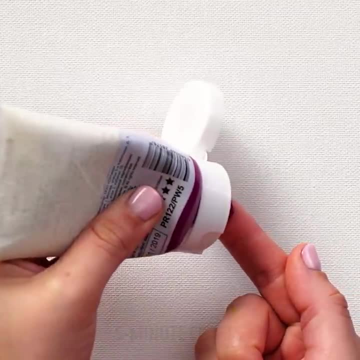 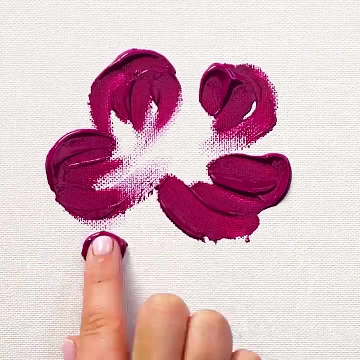 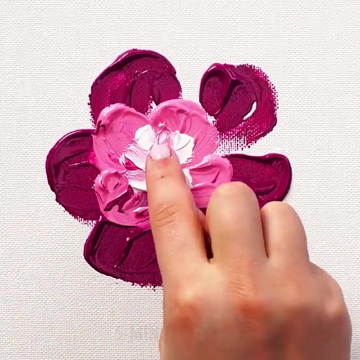 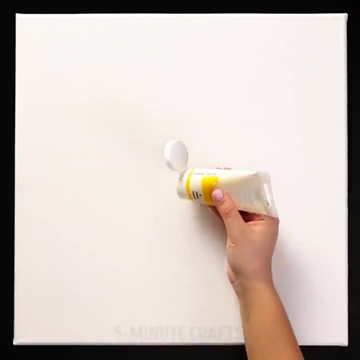 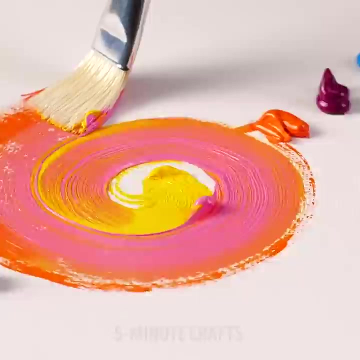 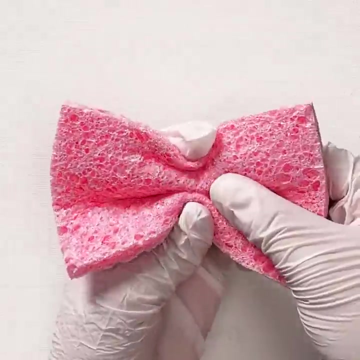 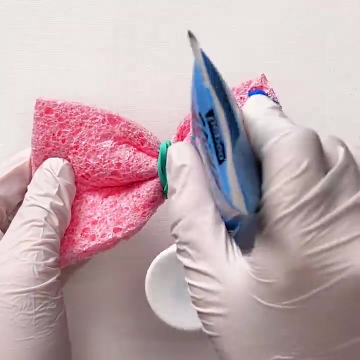 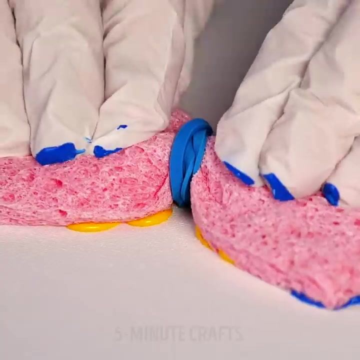 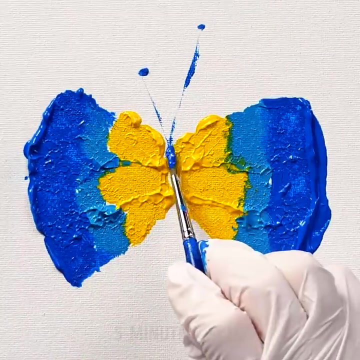 Nothing's gonna save us from our doubts, Nothing's gonna make us spell it out. I don't wanna be the one to say, oh, I told you so, But I told you so, But I told you so. I might be broken down, but I'm smiling. 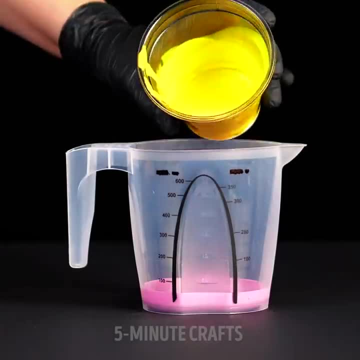 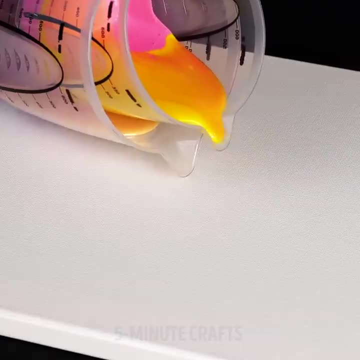 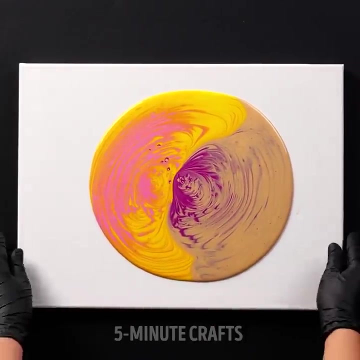 I keep my head up high, though I fail. Sometimes I get a bit emotional, But then I turn around and let it go. I see you watching me from a distance. I see you can't decide what to feel, But if you dig a little deeper, boy, 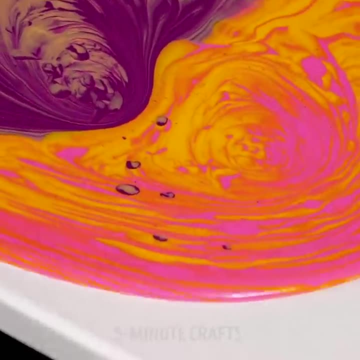 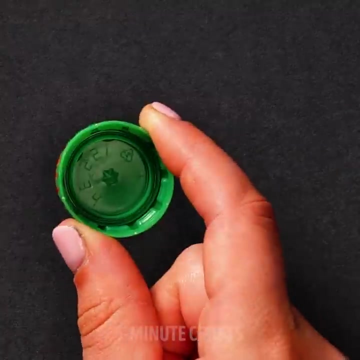 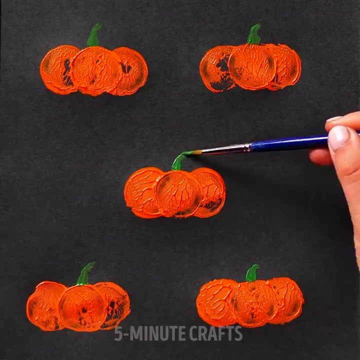 You know you really wanna get to know me. Let's get this out of the way. I can't wait. I don't know what to say. To tell you you shouldn't wait. Don't be so afraid. Yeah, I'm a bit too much, but I'm finding it.